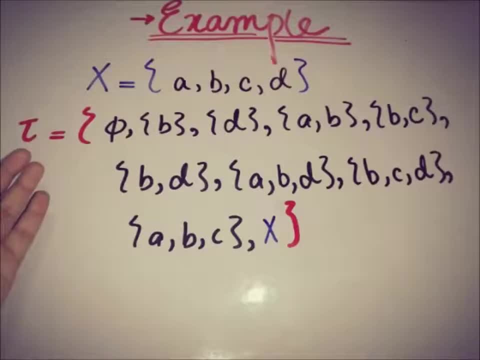 elements are here and the collection of subset that is tau and that is a topology having elements empty set b, d a, b, b, c, b d a, b, d, b, c, d a, b, d, b, c, d a b. 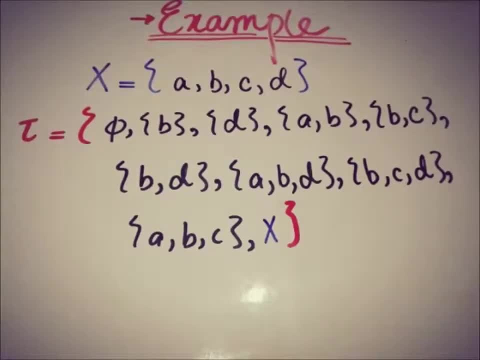 c, d, a, b, c and the space x or the set x. So this is a topology on the space x and we can prove this, that it is a topology on the space x, by proving the very three basic properties of being a topology on set x. The very first property is that of the existence. 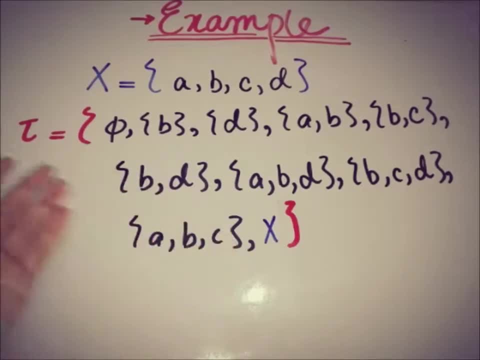 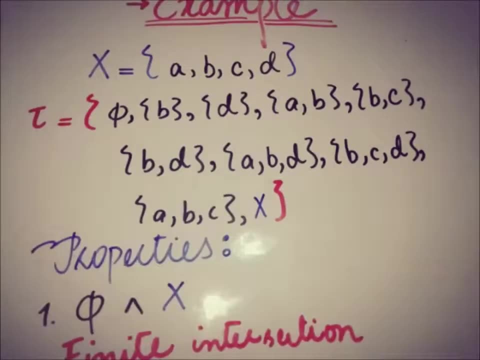 of the empty set and the space x or the set x in the collection of the subset of x and taken one is of. the second is a finite intersection and this is depend upon the number of elements that was present in the collection of subsets of x, So we can take finitely many elements. 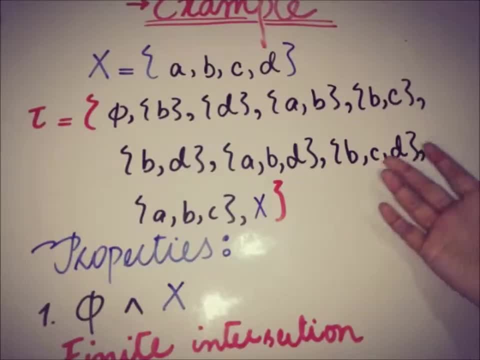 from this collection, tau, and we'll check whether the answer will be in this tau or not. So you can check now that whether taking the finitely many elements from tau will be in tau. So the third property of being a topology is arbitrary unions, and talking about the 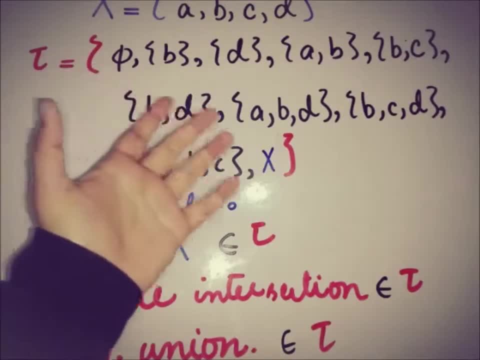 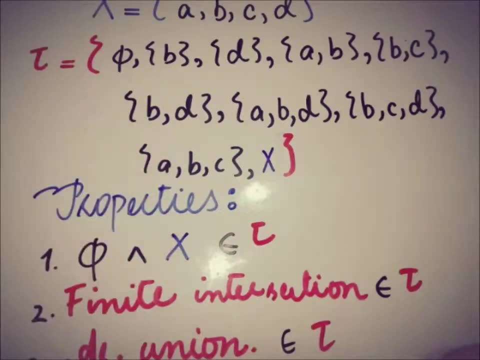 arbitrary union, that is, taking the arbitrary unions of some of the elements or whatever you want from this collection and we'll check that whether the union will be in that collection as well or not. So this is the right example of checking that, whether this collection is. 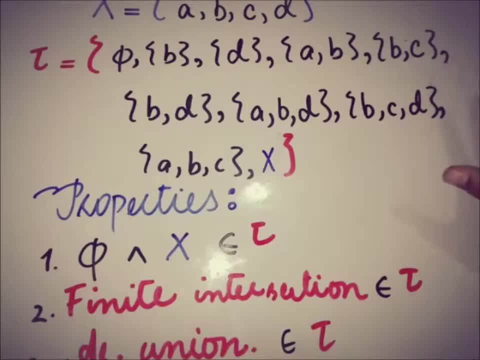 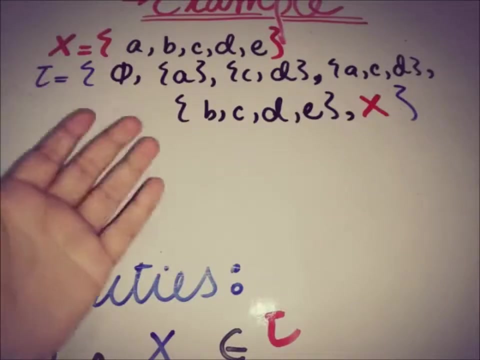 a topological space or not. and this is a topology, So you can verify this by these three properties. And the other example of topology is now we have a space. x contains abcde as elements and the collection of subset of x, ie tau. 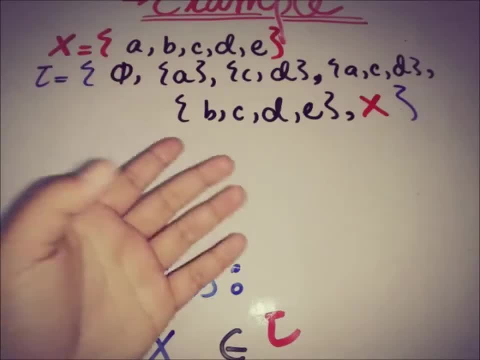 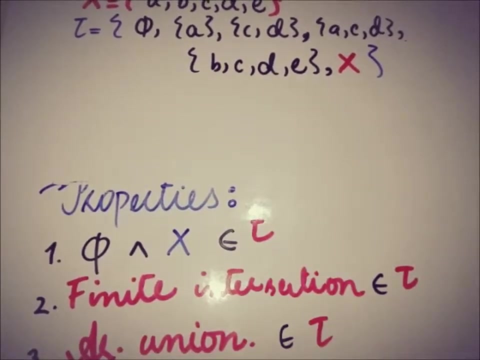 that is also a topology on x. have empty set, set, adc, acdbcde and the set x as well, a topology on the set X by the help of these properties, the very first of the existence of empty set and X. the second is a finite intersection and the third